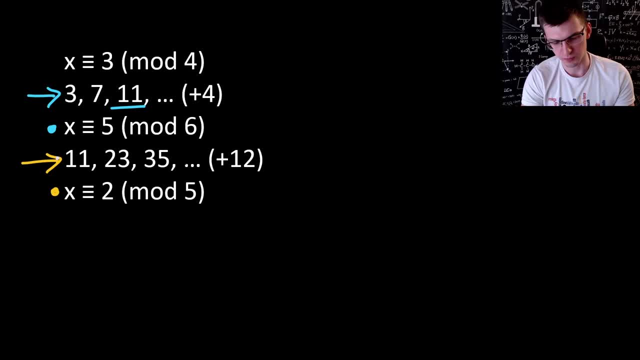 Apparently, I need some bigger value. after 35 plus 12, that's 47, and 47 modulo 5 is 2. indeed, This is the smallest solution for our system of three congruences, Again not the only one. We can increase it by what By least common multiple of 4,, 6, 5.. All moduli values. 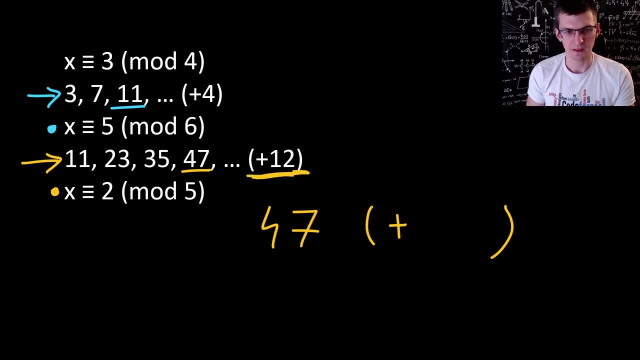 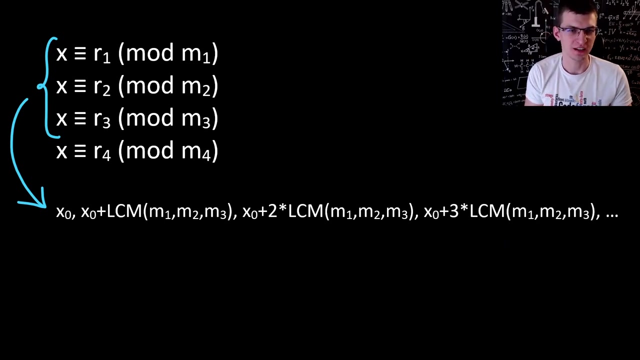 It's easiest to compute it by taking the previous LCM and the new modulus value and just grabbing those two, computing their LCM. In this case that's 60. Smallest value divisible by 12 and 5.. But then there's 107,, 167, 227 and so on. This method still works if there are more congruences. 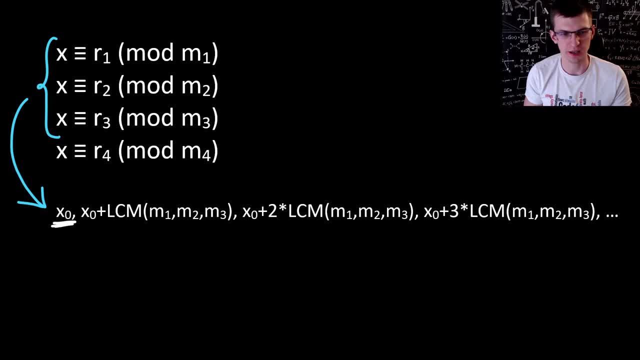 Let's say that you found solution for first three congruences x0 and you computed least common multiple of the first three moduli LCM of this. Then here is the sequence of solutions for first three congruences and in this sequence we need to find the first value satisfying the fourth congruence. 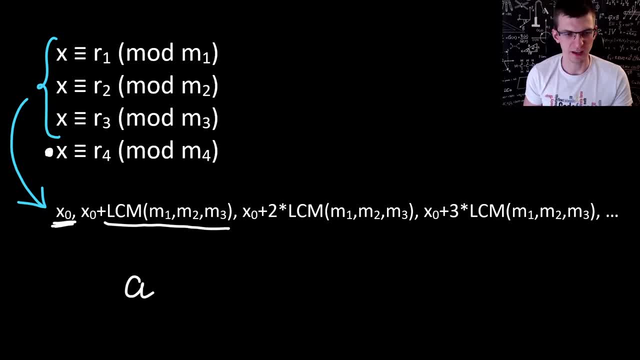 After we find it, let's say it's a, you can keep increasing it by LCM of all four moduli. and now, instead of going one by one through them again and computing least common multiple, let's use the fact that we already know LCM of this. Well, we used it here. It was that previous number plus. 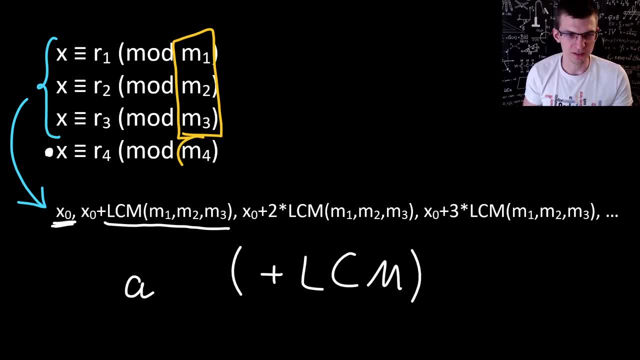 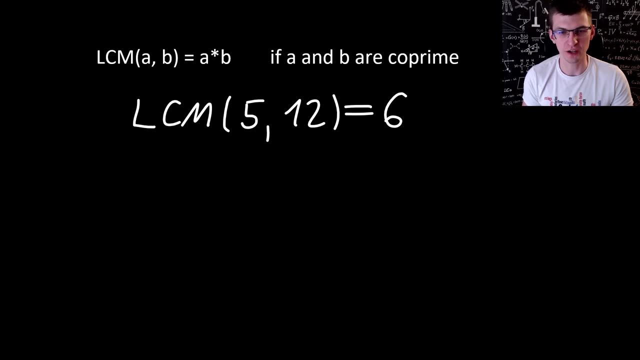 in brackets and we compute LCM of this and modulus 4. Then the sequence of available solutions is a a plus LCM, plus twice LCM. If moduli are co-prime, then their LCM is simply the product. like for 5 and 12, it's just 60,. 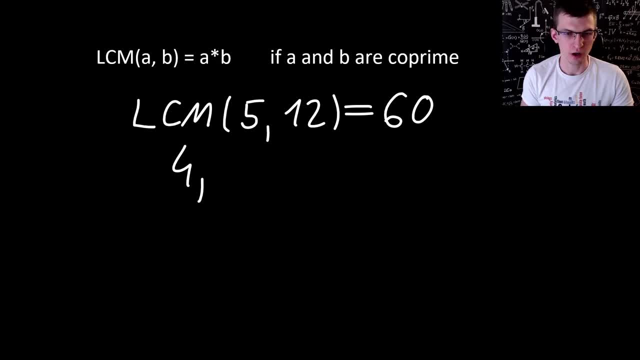 but it doesn't work. if there is some common divisor For 4 and 6, their product is 24 and yet there is smaller multiple, 12.. If you use product instead of LCM, you would miss some values and maybe also the solution In the previous example. you would have 11, maybe increased by 24 multiple. times. That's a sequence: 11,, 12,, 13,, 14,, 15,, 16,, 17,, 18,, 19,, 20,, 21,, 22,, 22,, 23,, 24,, 24,, 25,, 26,, 27,, 28,. 29,, 30,, 30,, 31,, 42,, 35,, 32,, 35,, 32,, 34,, 35,, 36,, 37,, 38,, 40,, 42,, 34,, 35,, 39,, 40,, 42,, 43,, 44,, 45,. 44,, 42,, 45,, 42,, 45,, 46,, 45,, 49,, 51,, 52,, 52,, 53,, 52,, 51,, 52,, 53,, 52,, 53,, 55,. 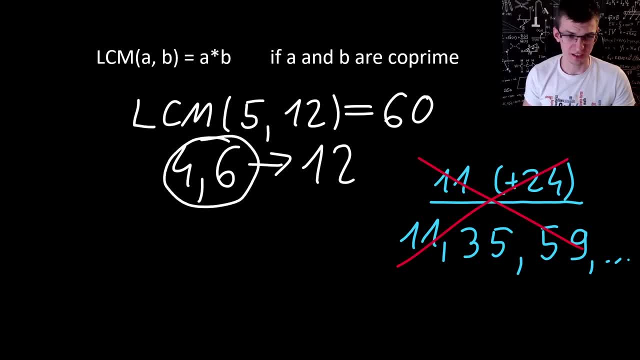 55,, 59 and so on, and you miss 47, which is solution for first two congruences. The easiest way to compute this LCM for two not co-prime values is to write down multiples of one of the two values, like 4, 8,, 12,, 16 and so on. Among them, find the first one divisible by the. 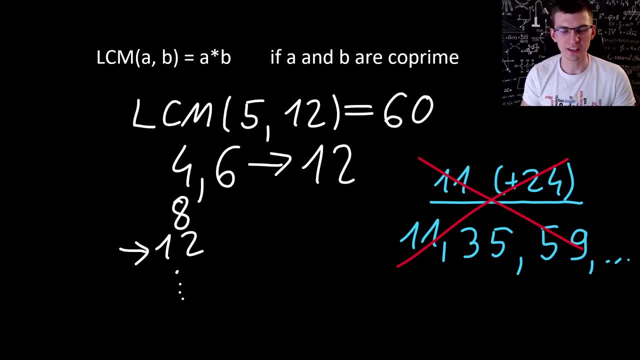 other value, 12 is divisible by 6,, so 12.. Either that or, alternatively, use this formula: LCM is product divided by the greatest common divisor of a and b. The common divisor of 4 and 6 is 2, so LCM is 24 divided by 2.. 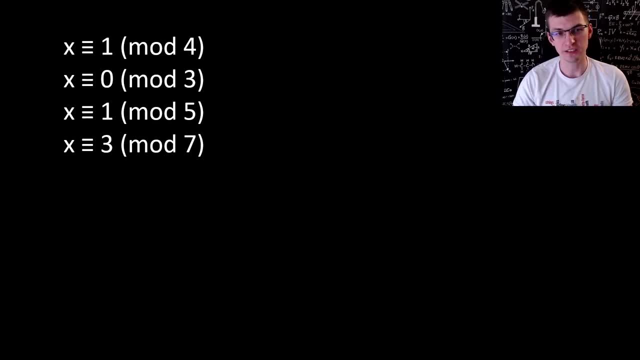 Let's solve this bigger example and learn two new tricks. The first one is that I can reorder congruences to make all the computations easier. When I see equal remainders, it's good to put them at the top, because I immediately see the solution for them. 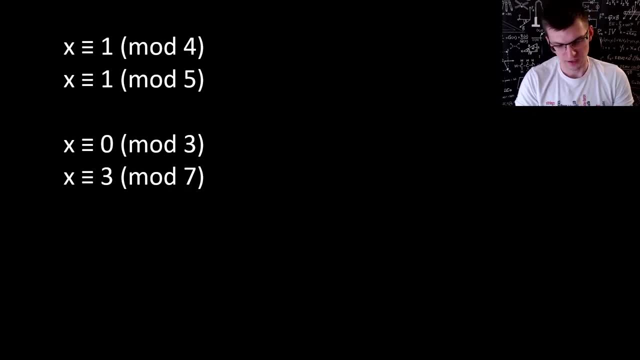 I put third congruence to the second spot, and I know that x equal to 1 works for the first two. Then it can be increased by LCM of 4,, 5, those are coprime, so just the product 20.. 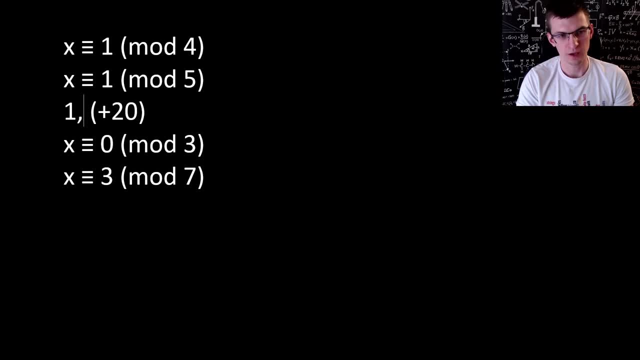 20 is divisible by both 4 and 5,, 1,, 21,, 41, and so on. This is a sequence of solutions for the first two congruences. Next step in this sequence: find the first value satisfying this, so divisible by 3.. 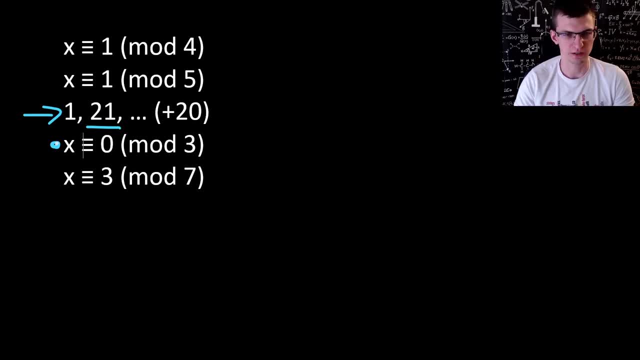 1 doesn't work. 21 does work. it is divisible by 3.. Here I have 21,, LCM of 20 and 3, they are coprime, so simply product I can increase by 60.. 60 is value divisible by all moduli so far: 3, 5, and 4,, 21,, 81,, 141, and so on. 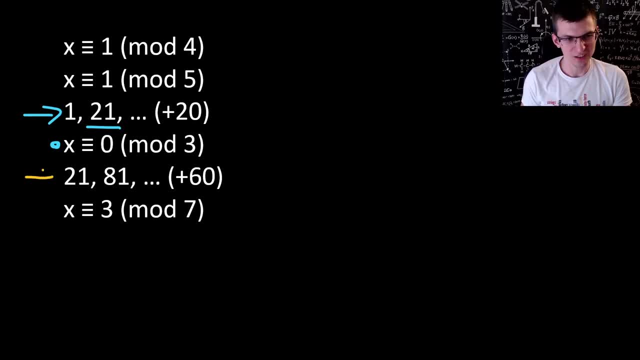 And the second trick will be useful. It's a little bit annoying to look at this whole sequence and find the first value satisfying this: 3 modulo 7.. 21 is 0 modulo 7, but then every next number gets more and more annoying to compute. 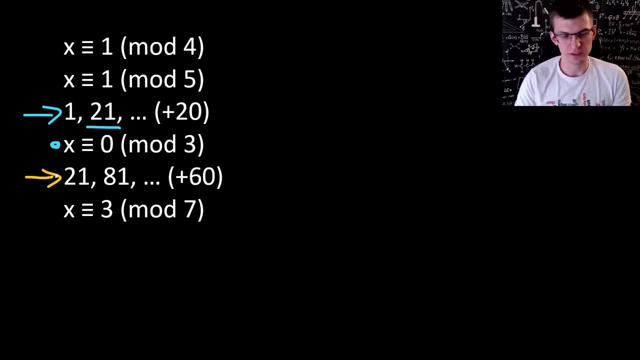 Instead of doing all that math, I'm going to do something smarter: 21 modulo 7 is 0, and 60 modulo 7 is what? 49, 56, I think it's 4 modulo 7.. Which means that, basically, I'm adding 4 modulo 7.. 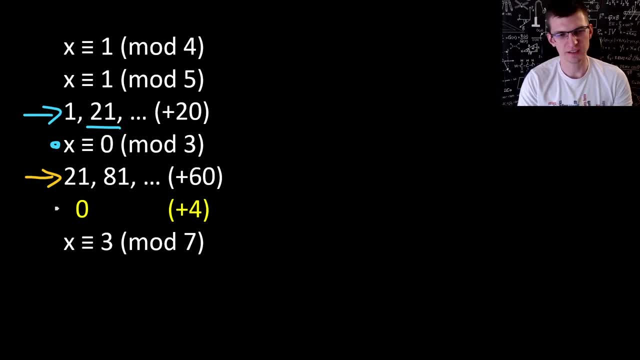 Instead of looking at this number, I can kind of forget about it and I can say that 0 plus 60 is like 0 plus 4.. So here remainder is 4.. Then the next one: 4 plus 4 modulo 7 is 1.. 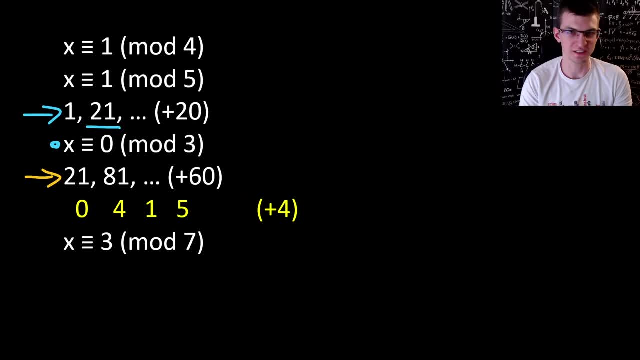 Then this plus 4 modulo 7 is 5, and so on. This is the second trick. You can just work with remainders to avoid computations with any big values: 5 plus 4.. So like 5 plus 60, simplified is just 5 plus 4, because 4 and 60 is the same modulo. 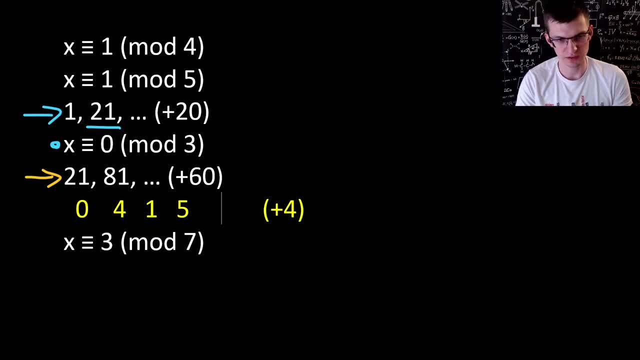 7.. 5 plus 4 is 9,. modulo 7 is 2, and I'm looking here for the first value, equal to 3.. 2 plus 4,, 6,, 6 plus 4,, 10, modulo 7 is 3,. alright done. 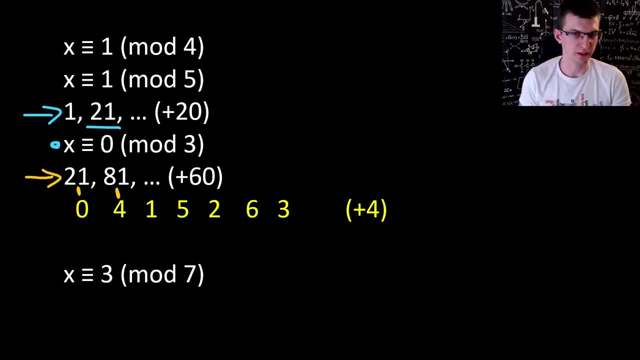 0 represented 21,. 4 represented 81,. 21 plus 60,. this is 21 plus twice 60, 3 times 60,. 4 times 5 times 6 times. this is 21 plus 6 times 60, 360, so in total 381, that's the. 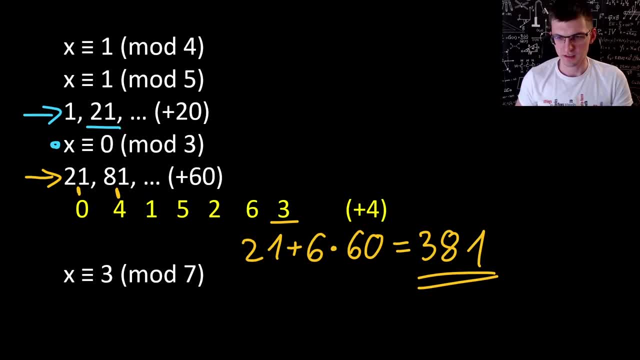 solution And if you want to find all the solutions- the new LCM is LCM of 60 and 7, 60 represented LCM of moduli so far- then also we need to consider 7, 60 times 7, 420.. Remember: if they are not co-prime, it's not simply a product. Remember: if they are not co-prime, it's not simply a product. Remember: if they are not co-prime, it's not simply a product. 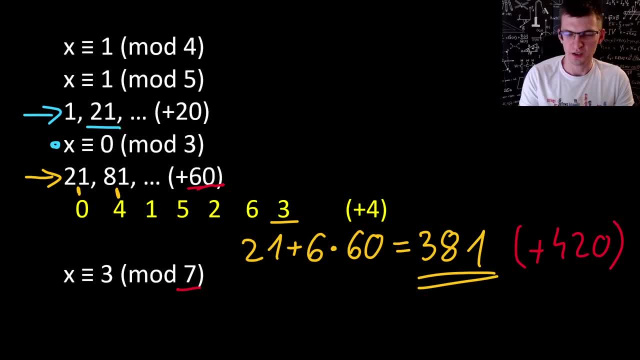 So the next solution is 381 plus 420, 801, I think, and so on. That was everything you need to know. but here is something extra. Look at this sequence of remainders. The next element after 3 would be 3 plus 4, 7,. modulo 7, it's 0, then 4, 1, and so.